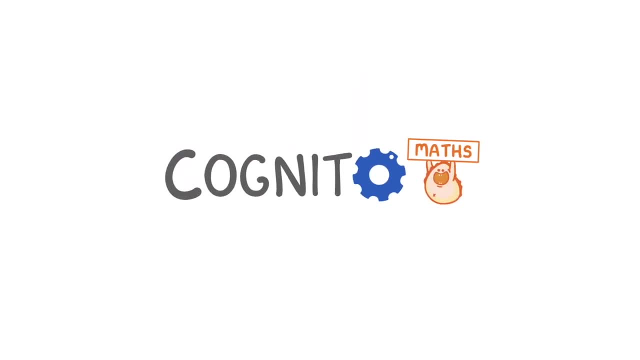 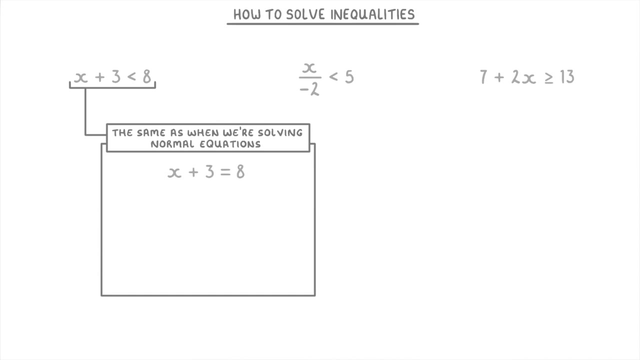 In this video we're going to cover how to solve inequalities like these three. The idea is exactly the same as when we're solving normal equations with an equal sign, So just like how we normally want to see the unknown letter by itself on one side of the equation. 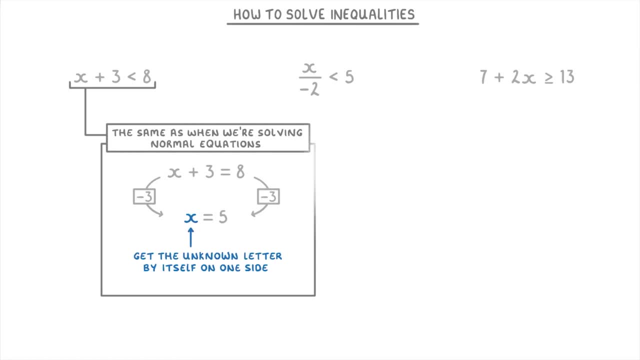 that's exactly what we're trying to do here as well. So in this first inequality, x plus three is less than eight. to get the x on the left by itself, we're going to have to subtract three from both sides to find that x is less. 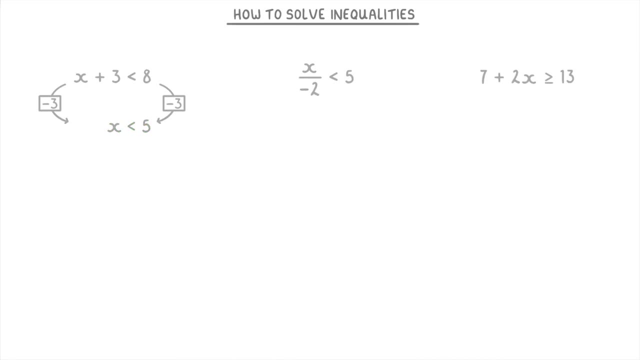 than five, And that's it. So, essentially, we treat the inequality sign as if it's an equal sign, but we don't actually change it to an equal sign. The only important difference that you need to know about is that if you multiply or divide both sides- 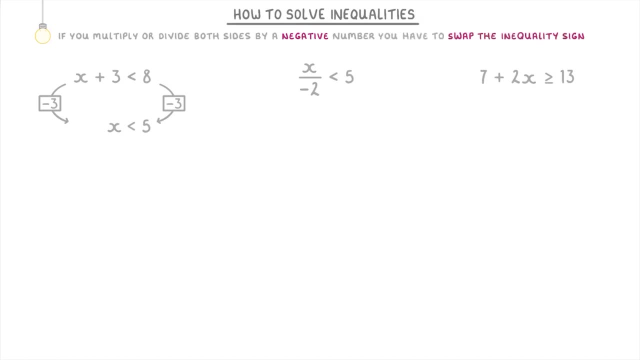 by a negative number, then you have to swap the inequality sign around. For example, in this second equation, to get rid of the divide by negative two part, we need to multiply both sides by negative two, which will leave us with just the x on the left and negative. 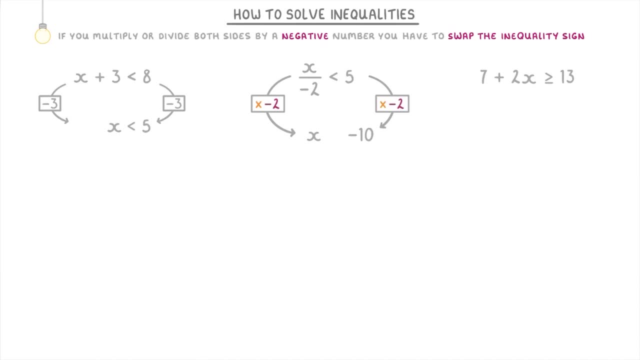 10 on the right. But, importantly, because we multiplied by a negative number, we're going to have to swap our inequality sign around so that it will change from a less than to a more than sign, which leaves us with x is more than negative 10.. 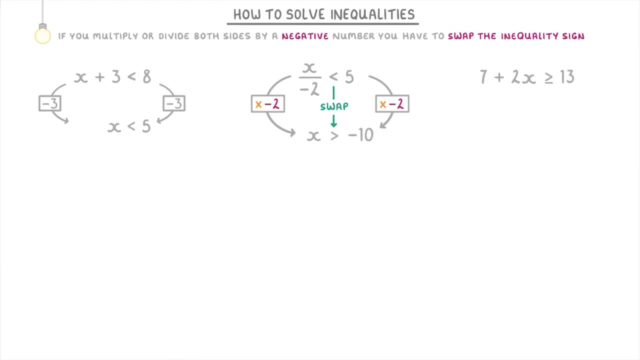 The last question here- seven plus two x is more than or equal to 13,- is a bit trickier because it involves two steps. The first thing we're going to have to do is take away seven from both sides to get two x is more than or equal to six. And then we're going to have 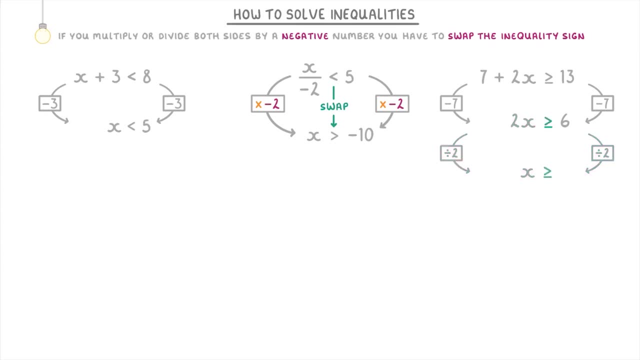 to divide both sides by two, To get x is more than or equal to three, And that's it. Let's try a couple more. For this first one, there are two different ways that you could do it. One is to subtract five from both sides to get minus three: x is less than or equal. 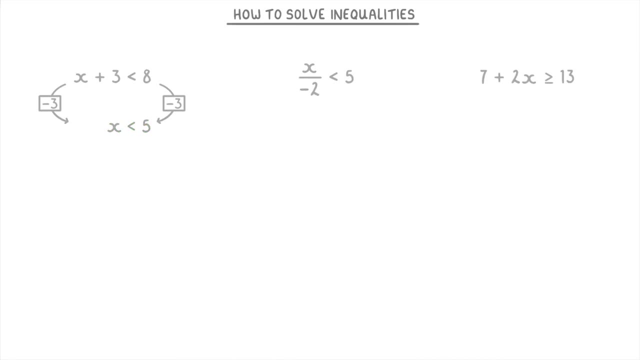 than five, And that's it. So, essentially, we treat the inequality sign as if it's an equal sign, but we don't actually change it to an equal sign. The only important difference that you need to know about is that if you multiply or divide both sides- 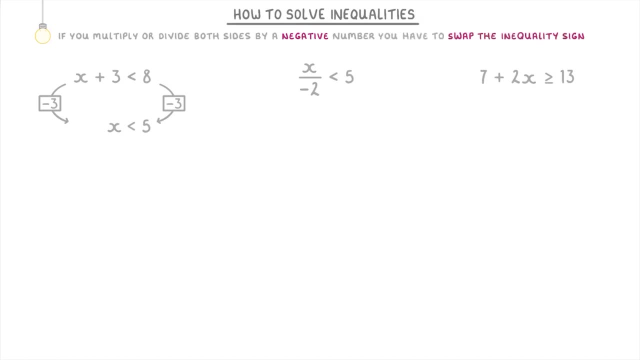 by a negative number, then you have to swap the inequality sign around. For example, in this second equation, to get rid of the divide by negative two part, we need to multiply both sides by negative two, which will leave us with just the x on the left and negative. 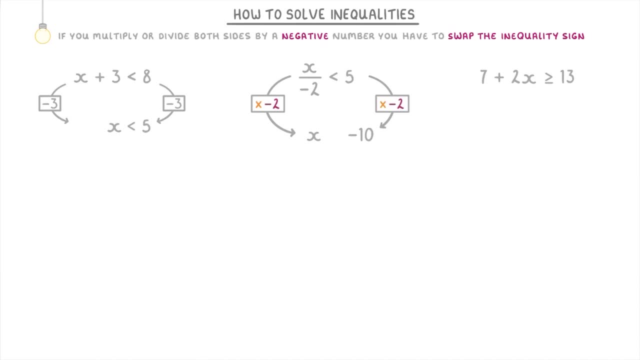 10 on the right. But, importantly, because we multiplied by a negative number, we're going to have to swap our inequality sign around so that it will change from a less than to a more than sign, which leaves us with x is more than negative 10.. 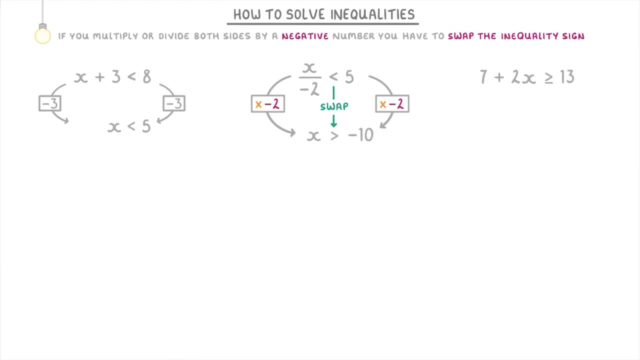 The last question here- seven plus two x is more than or equal to 13,- is a bit trickier because it involves two steps. The first thing we're going to have to do is take away seven from both sides to get two x is more than or equal to six. And then we're going to have 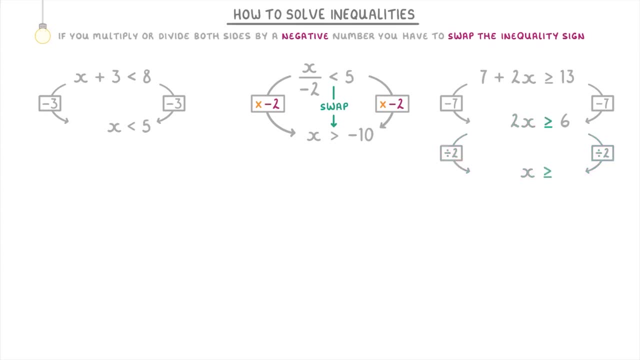 to divide both sides by two, To get x is more than or equal to three, And that's it. Let's try a couple more. For this first one, there are two different ways that you could do it. One is to subtract five from both sides to get minus three: x is less than or equal. 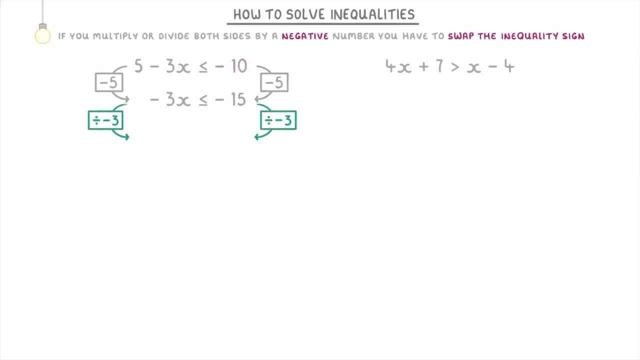 to negative 15.. And then divide both sides by negative three to find that x is more than or equal to 5.. And if you didn't notice, we swapped our inequality sign around here because we were dividing by a negative number. Then the second way that we could have done this 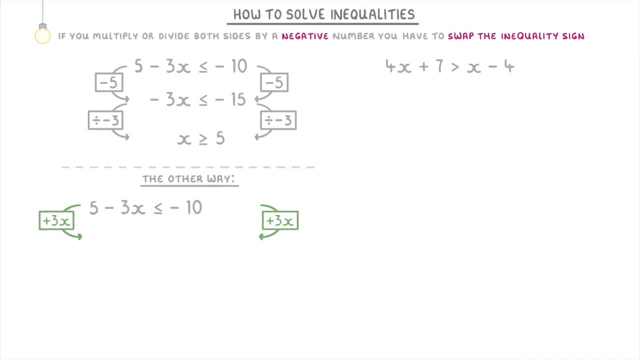 question would be: to add 3x to both sides to get 5 is less than or equal to negative 10 plus 3x. then add 10 to both sides to get 15 is less than or equal to 3x. and finally, 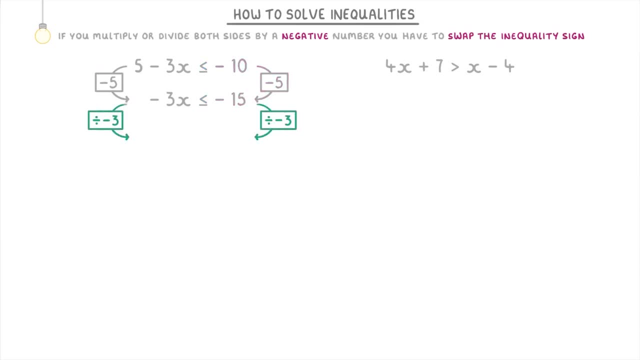 to negative 15.. And then divide both sides by negative three to find that x is more than or equal to 5.. And if you didn't notice, we swapped our inequality sign around here because we were dividing by a negative number. Then the second way that we could have done this 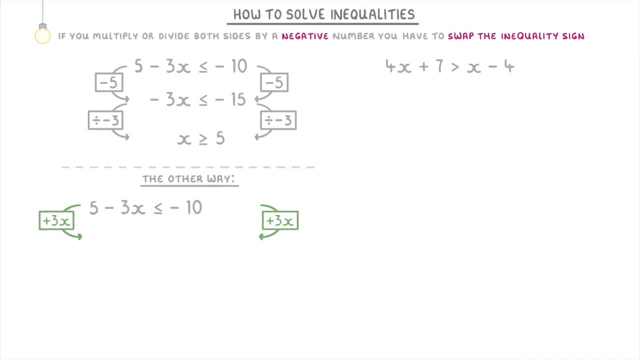 question would be: to add 3x to both sides to get 5 is less than or equal to negative 10 plus 3x. then add 10 to both sides to get 15 is less than or equal to 3x. and finally, 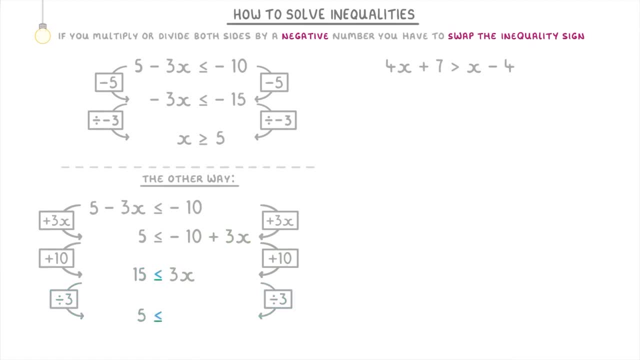 divide both sides by 3 to get 5 is less than or equal to x. And remember, this is exactly the same thing as saying that x is more than or equal to 5, like we got in the first place. In situations like this, it doesn't really matter which way around you do it. 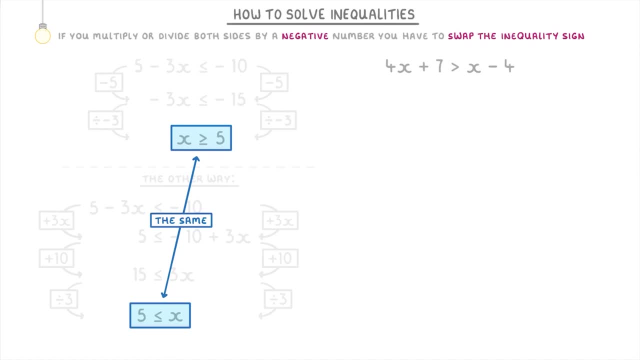 Just go with whichever one you feel most comfortable with or whichever one you think of at the time. For the second question, there are also two ways of doing it, because we could try to put the x's on the left or the right, But because at the moment there are more x's. 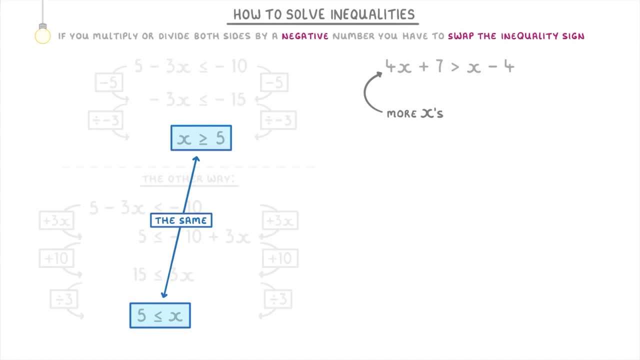 on the left hand side, it'll be better to keep our x's on the left and put our numbers on the right. So the first thing you do is subtract x from both sides to get 3x plus 7 is more than negative 4.. Then you can subtract 7 from both sides to get 3x is more than negative. 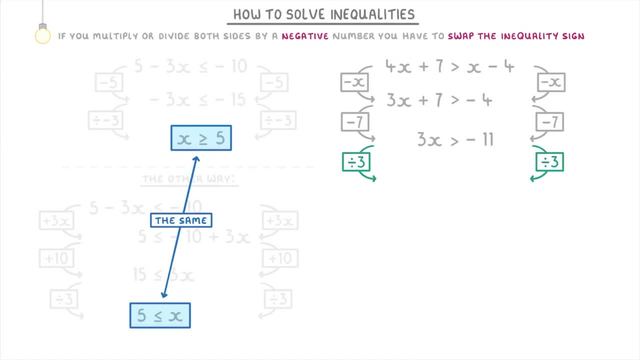 11, and finally divide both sides by 3 to get x is more than negative 11 over 3.. And we can leave our answer like that, because we can't simplify negative 11 over 3.. Anyway, that's it. 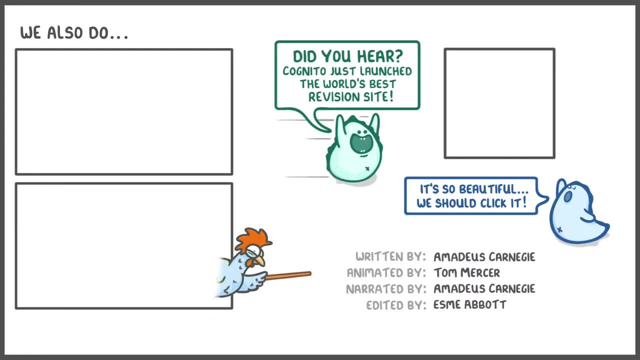 That's everything for this video, So hope that all made sense. If you enjoyed it, then do give us a like and subscribe, and cheers for watching.